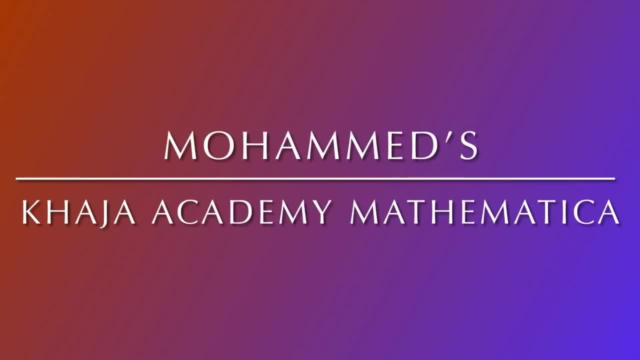 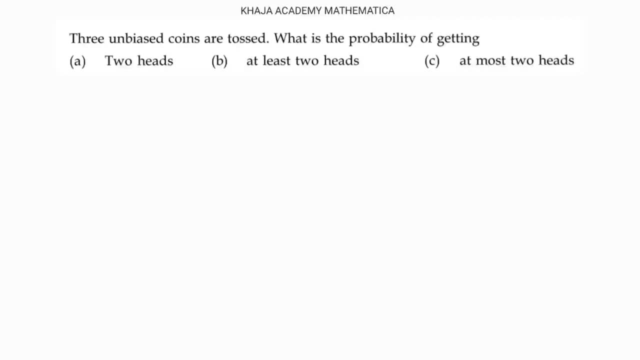 Three unbiased coins are tossed, what is the probability of getting two heads, at least two heads, at most two heads now here, when three coins are tossed? see the possible outcomes. see, if you write like this- it will be easy right now: four heads, then write four tails, then write two heads, two tails, then again write one head, tail, head, tail, head, tail, one one. so if you write like this, these are the possible eight outcomes. so this is eight outcomes, this one. 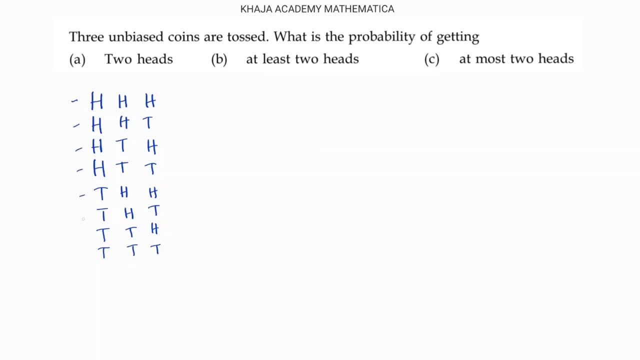 head, head, head, head, head, tail. like this you'll get all possible eight outcomes. now they're asking what is the probability of getting two heads. so probability of an event formula is: probability of an event is number of favorable outcomes. number of favorable outcomes by total number of outcomes. by total number of outcomes. 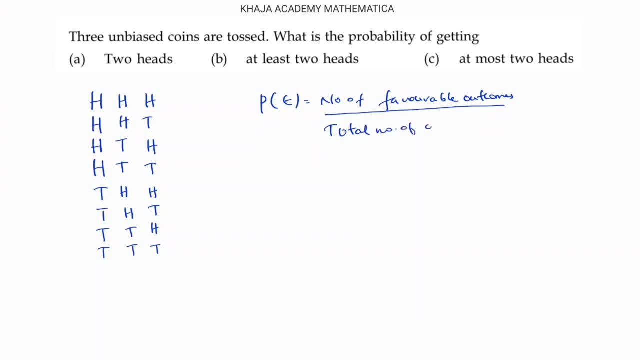 So here probability of two heads, probability of two heads, total outcomes are here eight. so two heads mean: see first, one we cannot take because here we have like three heads. second one we can take because it has exactly two heads. and third one, also two heads, here only one head and this one, so tail, head, head. so total three cases. so this is one head, head, tail. 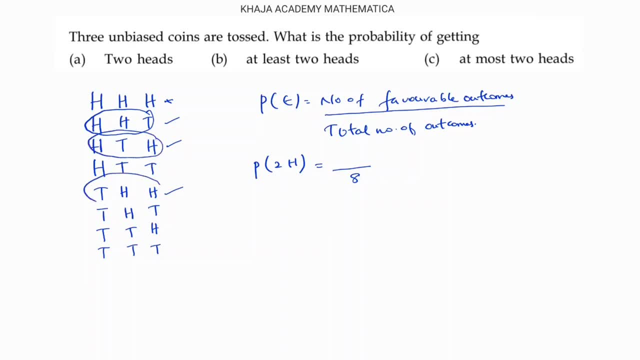 head, tail head and tail head, head. in these three cases we have two heads, so the probability of getting two heads is three by four. those are one, two and three, so the answer is three by sorry- eight. total eight comes up. total outcomes are eight. next probability of at least: 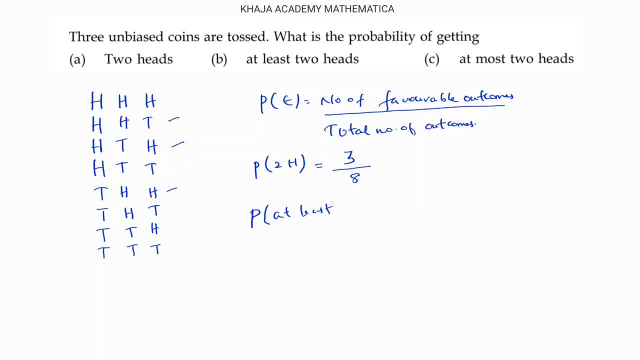 at least they are asking like two heads, probability of at least two heads. at least two heads see at least two heads. total outcomes are eight. so at least two heads means minimum two. so maximum you can get more than two also. so two and three. so here maximum is three, only. so two and three we can consider. so two and three. so if we 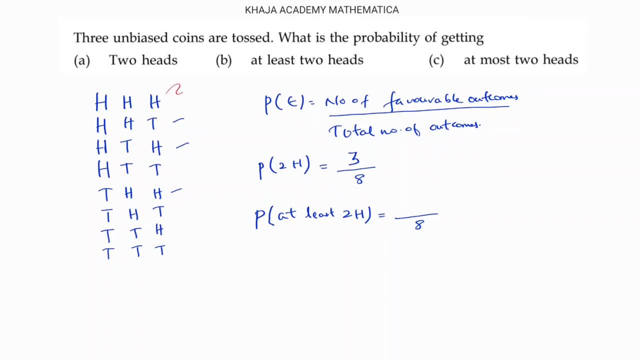 will see here. in the first one i can take this because here we have like three heads. i can take this one because two heads, this one also and this one because this case i cannot take because only one head is there, because at least two means two are more than. 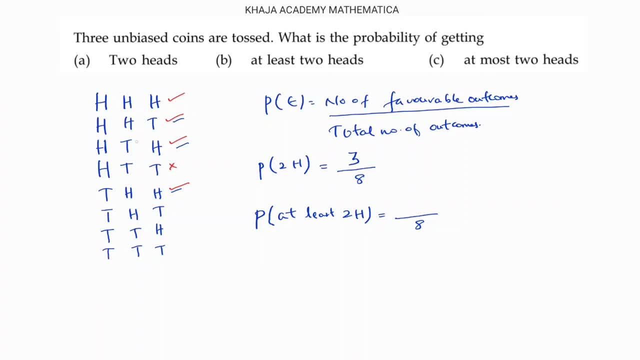 two, so this one head head, so this head head. so we take one head made two and head hair, so on this one head head, here also head, and head, here also head head, and here at least it also, we can take three also. so the answer is like one, two, three, four, four by eight, which is nothing but one by two. now, 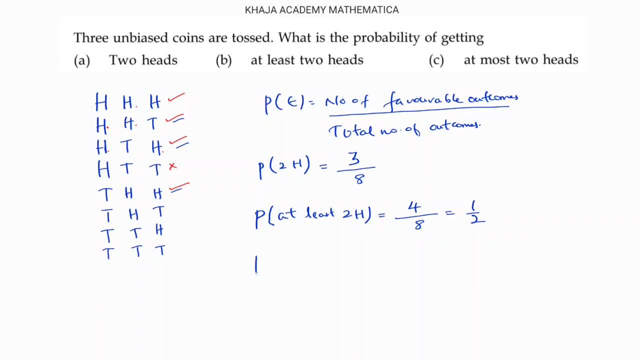 what is the probability of at most two heads? probability of at the most two heads. so again, total outcomes: eight. so now, at the most means, now see here, see, i can take at the most two head means you can take, get two, one, and if you not get head also, it's fine, that also you can. 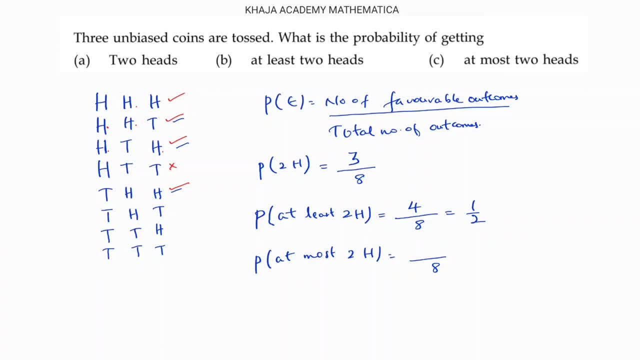 count, but it should not cross two, it should not cross two, which should not be more than two. so see here, in the first case it is three. i cannot take that. i can take this two heads case. i can take this also. i can take one head also two heads. 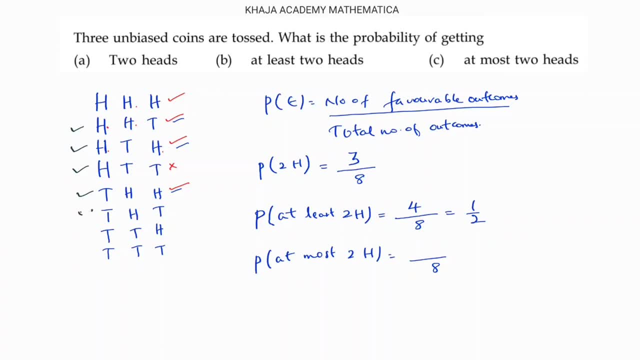 and here one head also i can take, because two i should not cross at the most. two means maximum is two, not more than two. so i can take this one and see the last one also i can take, because here zero heads, because i should not get more than two, means if you will not get also, it's fine.